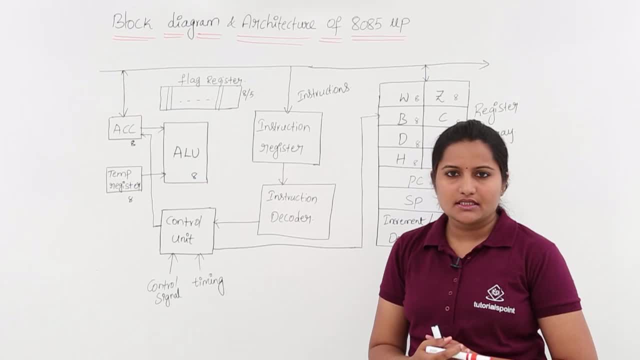 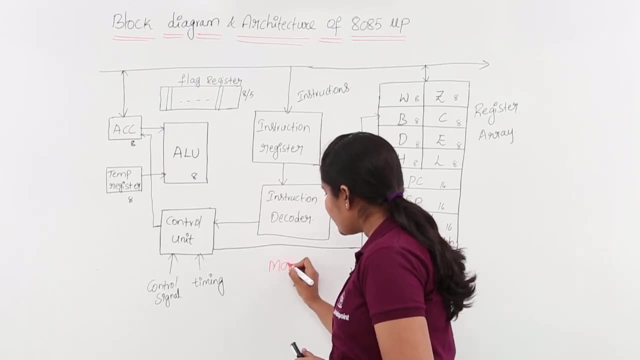 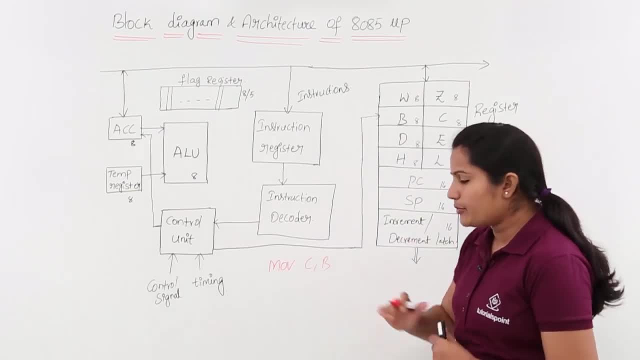 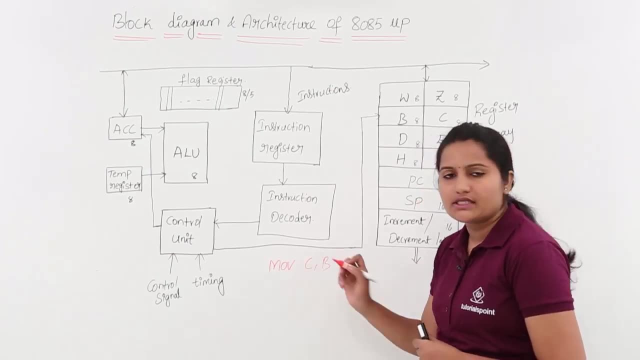 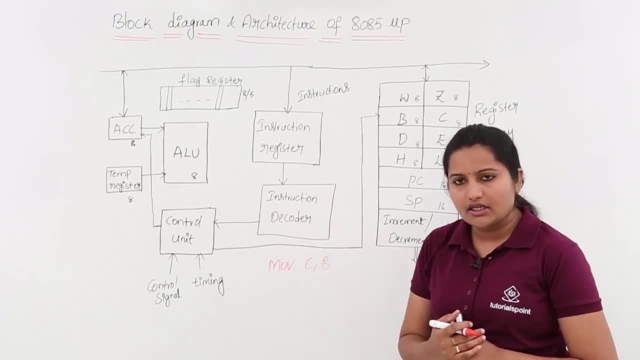 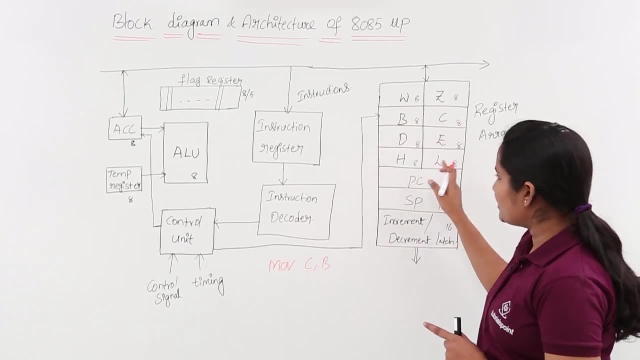 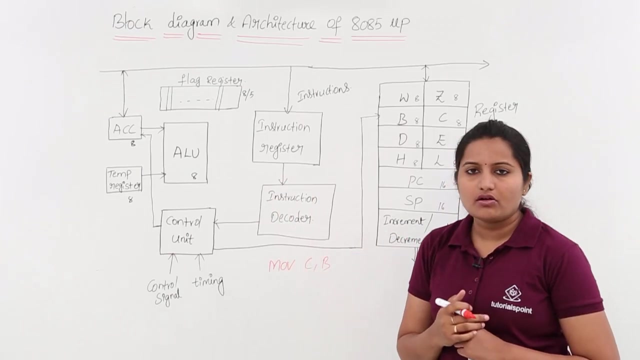 is stored in register and decoded instruction decoder and executed by control unit. here And now, coming to BC DE HL, All these are registers of 8 bits. that means BC DE HL and accumulator. all these are 8 bits, so these are called as. 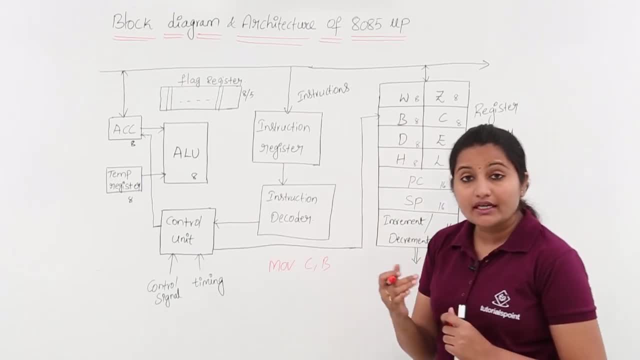 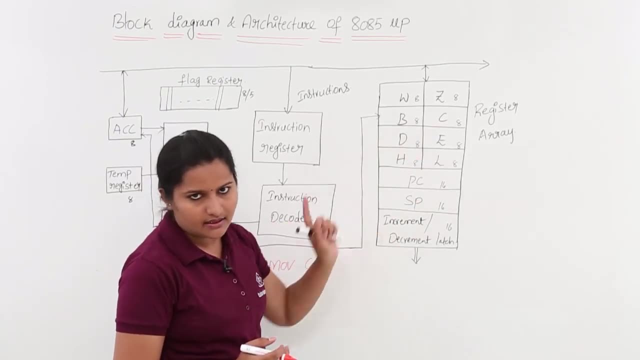 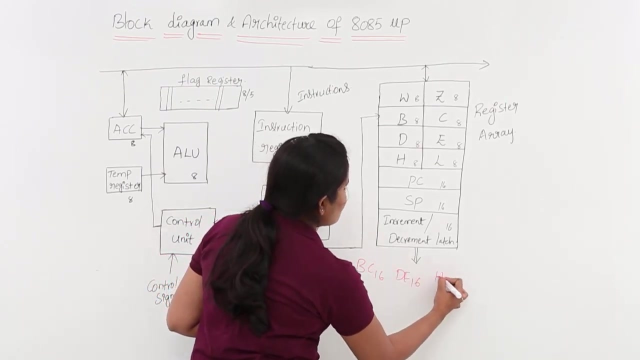 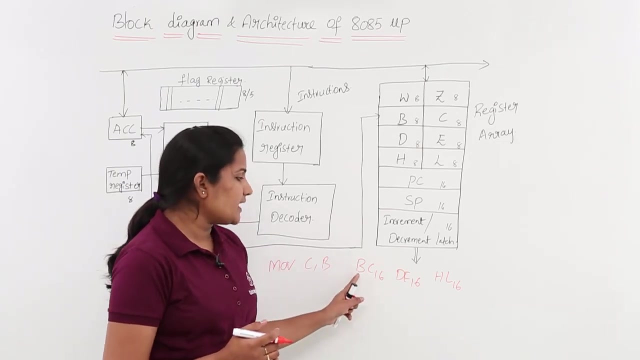 resistor pairs. where HL 16, when we return in pair, we need to write as 16 as suffix. when we take in separately, then we need to write 8, for example BC 16, so DE 16 and HL 16. this pair combination is very important. which resistors are pairs? so, for example, they given BD. that 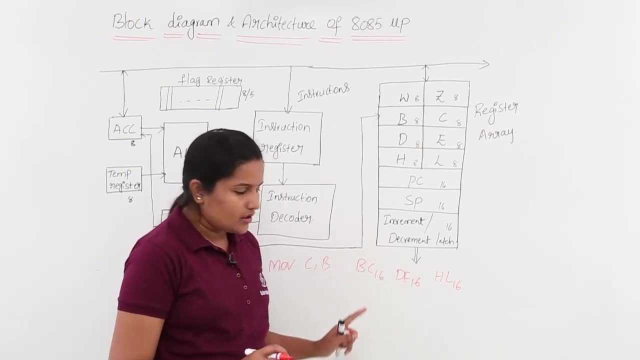 is not right if they given BH. that is not right. only BC is pair of resistor and DE is one pair and HL is one pair. combination is very important. so HL 16 is also used for memory pointing. that means this will acts as memory pointing resistor. 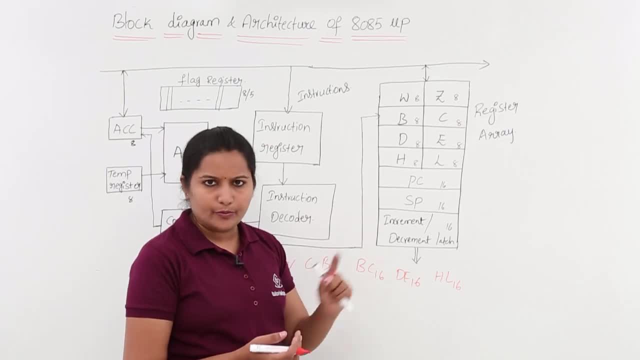 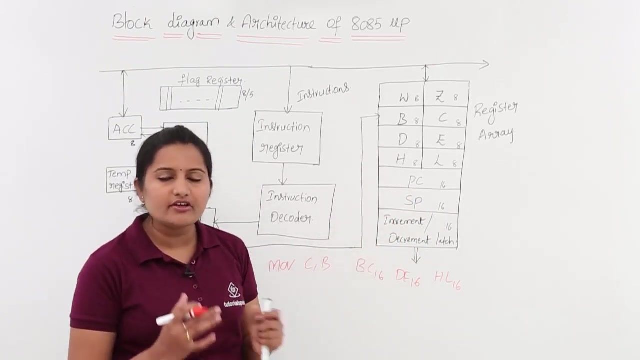 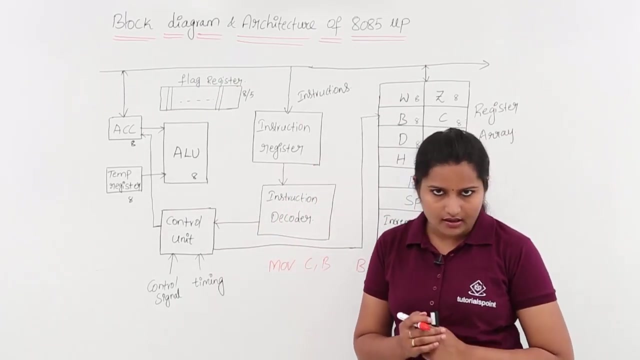 So here PCHL, PCHL and ASP program counter and stack pointer are used at special purpose resistors, and increment and decrement latch or counter is of 16 bits. so all these 3 are 16 bits register in our architecture. So the most important points that we may get as questions in technical exams are so: 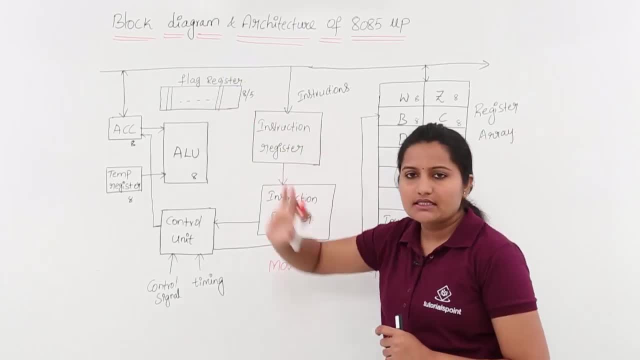 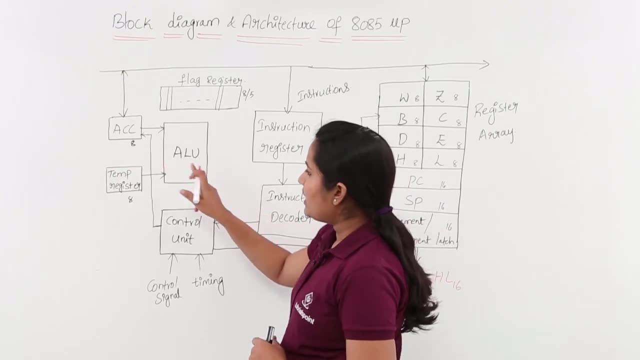 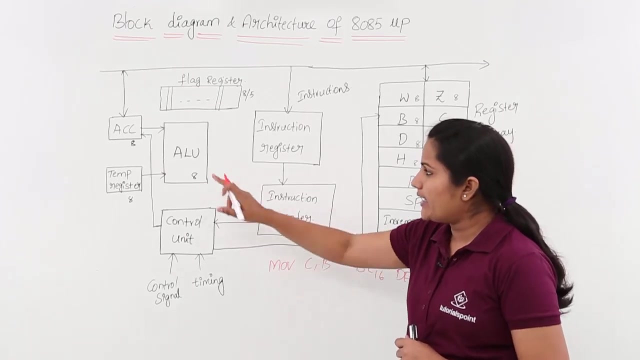 the architectural units and about flag resistor, how many bits are used? generally we will use 5 bits, 5 bits, even though that is of 8 bits, and here accumulator, ALU, that number of bits we need to mention accumulator or of 8 bits and ALU is of 8 bits, and here we are having register.